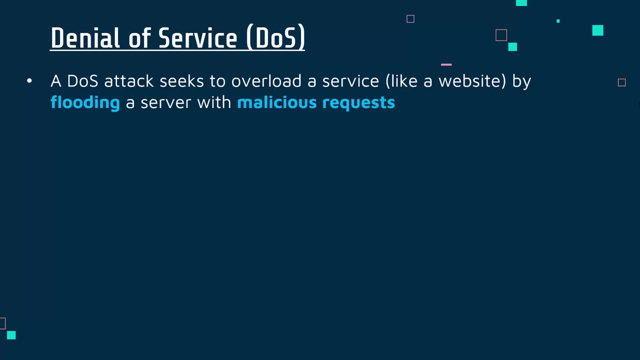 And so here the attacker is just doing loads and loads of these requests, trying to flood, trying to overload the server, So it stops working. to give you an example of how this might go, Let's say we've got Alice, who is our perfectly fine authorized user. She's allowed to access that, say, Microsoft. 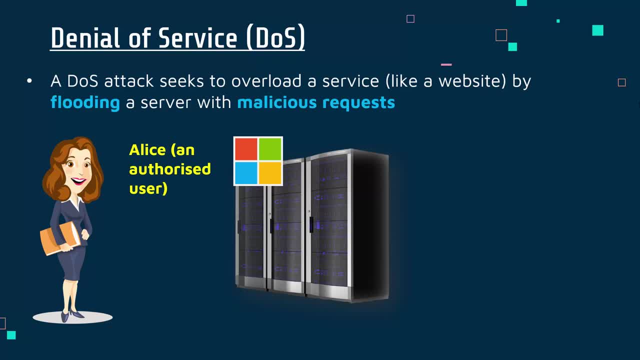 So Microsoft have got servers- Let's say these are web servers, servers being our really powerful computers which hold Information and give information to clients. So Alice wants to access Microsoft's website. say so, she requests access to this web page and the server has got no issue. 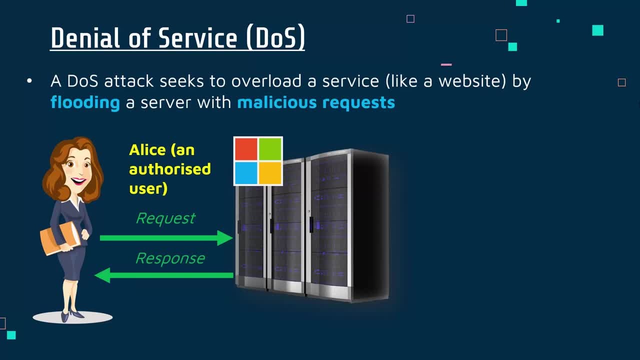 It gives it back and responds to her with the web page. That's how this communication should go. but if we've got a DOS attack happening, But let's say we also have a denial of service attack going on by somebody called Mallory, who is our attacker? 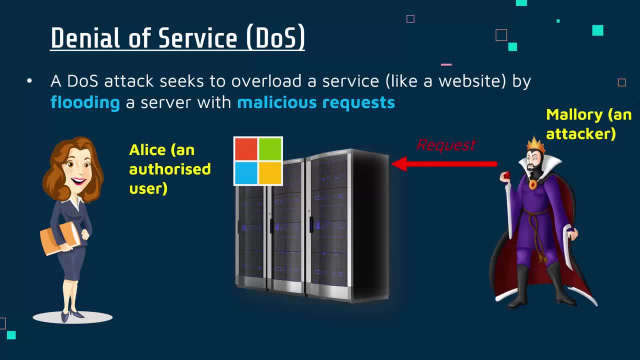 He's going to request the same information Alice did, but he doesn't care, He doesn't want the website, He's just trying to overreact. He's trying to overload the service, but Microsoft isn't to know this initially, So they will just respond as normal with a legitimate message giving the web page to him. but he doesn't stop there. 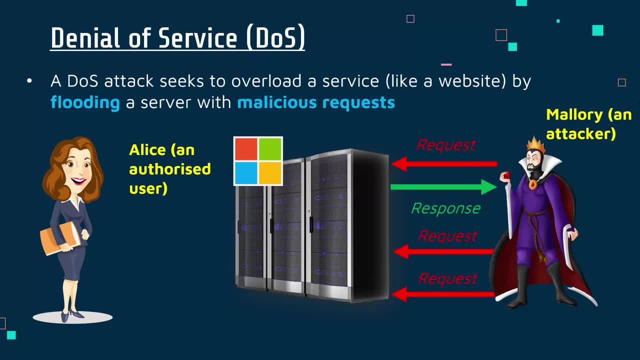 He's not going to just accept This. is going to keep requesting loads and loads of times, Maybe hundreds of times per minute, or even a quick of miss, if it's able to. I miss can if the server is not very powerful and hasn't got protection. 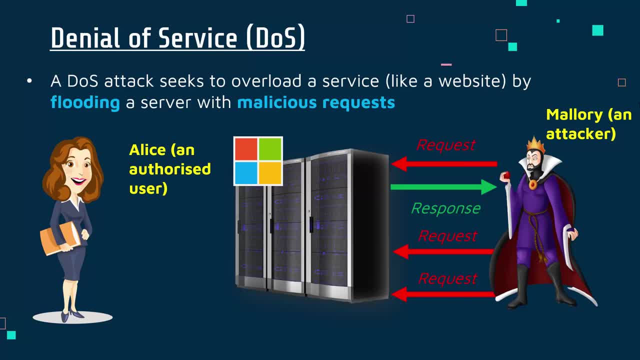 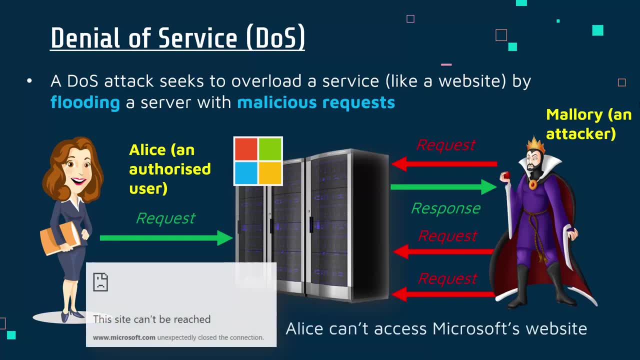 May and they may cause it to crash. it may not be able to Fulfill any of the requests coming from Mallory or from anybody else, So Alice might request it again and this time she might get a response saying actually you can't have it, or possibly even no response. 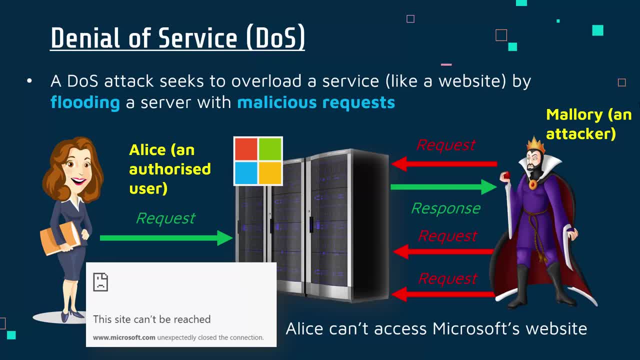 But just because Microsoft servers are overwhelmed because of this denial of service attack and the consequence for Microsoft or the company being affected Is they're not able to function normally, it disrupts their operation, It denies service to their legitimate users and so they can't make money, or it causes inconvenience, and so on. 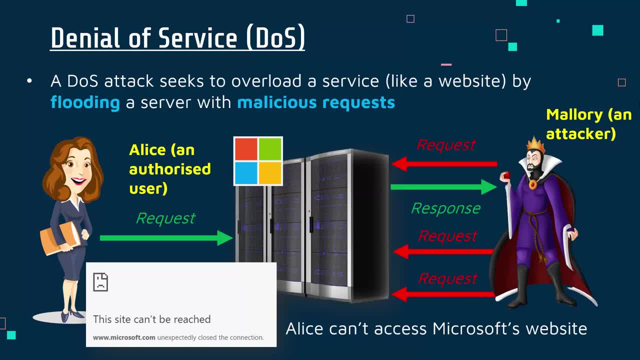 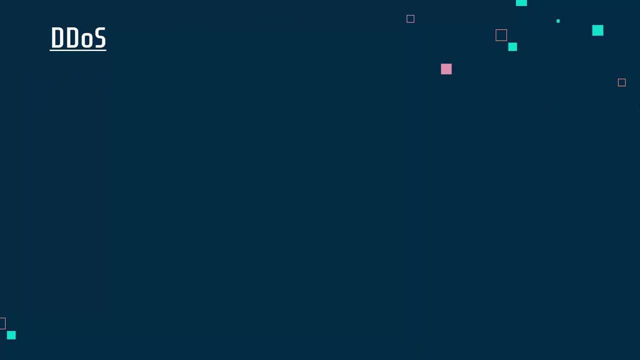 It causes issues for the organization. So there is a slight extension Of a DOS attack. a DOS attack which is a DDoS, which you may have heard of, especially if you do gaming or watch streamers and so on. it's a fairly common, unfortunately, attack. so a DDoS is.